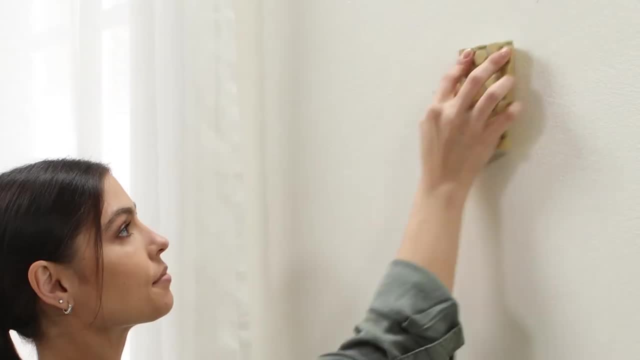 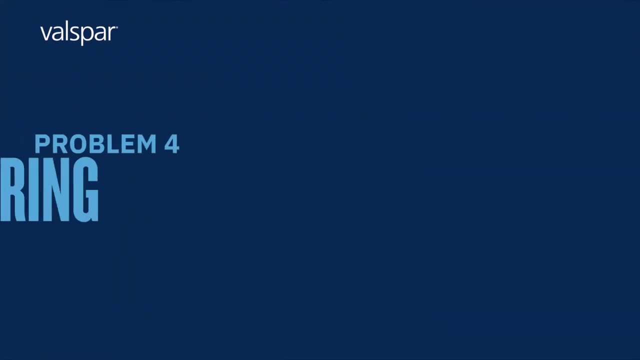 sharp scraper until it is fairly even with the wall. Then sand down with a fine grit sandpaper until the surface is light and smooth. Then sand down with a fine grit sandpaper until the surface is level and smooth. Now all you need is a little paint. 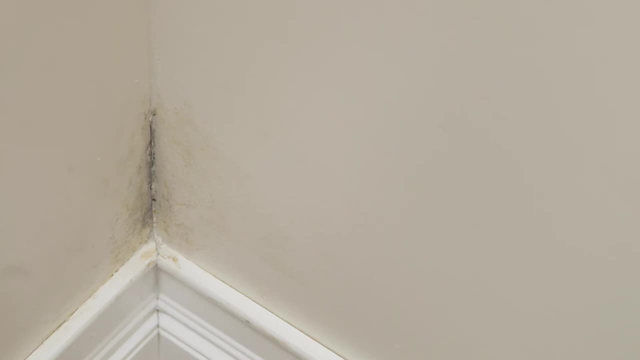 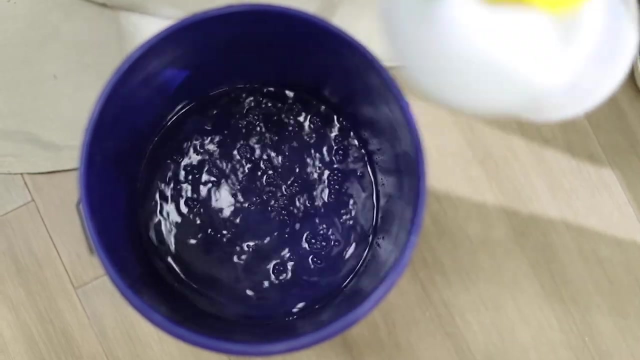 Now for removing mildew stains. There's a few more steps involved. You can effectively remove mildew or mold from the walls with a bleach and water solution and with the proper personal protective equipment like a face mask, safety glasses and gloves. First assess the condition If the wall 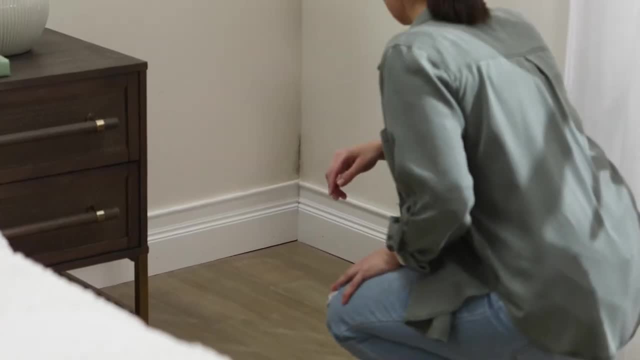 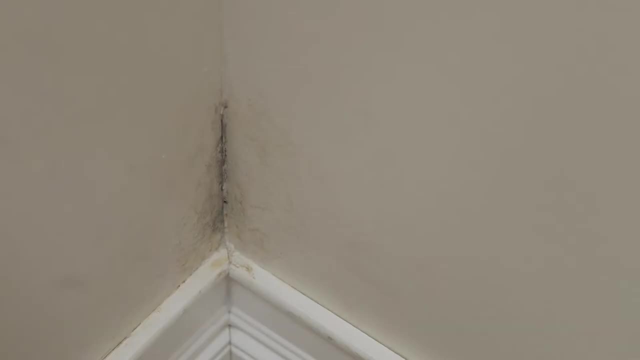 is beyond recovery, then it must be replaced. If you're unsure, ask a professional. Mold letters, untreated, can be extremely harmful to everyone in the home. If the wall surface is still functional, you should be able to remove the spots with a bit of elbow grease. Prep the area by covering. 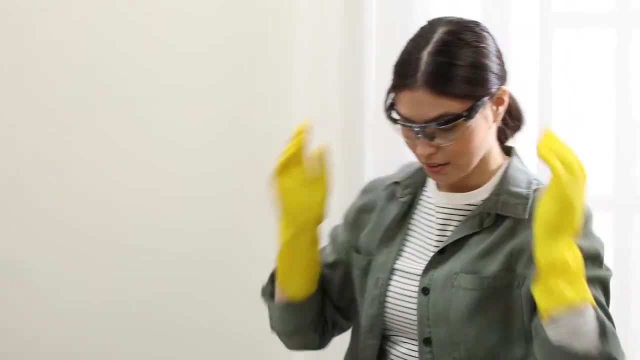 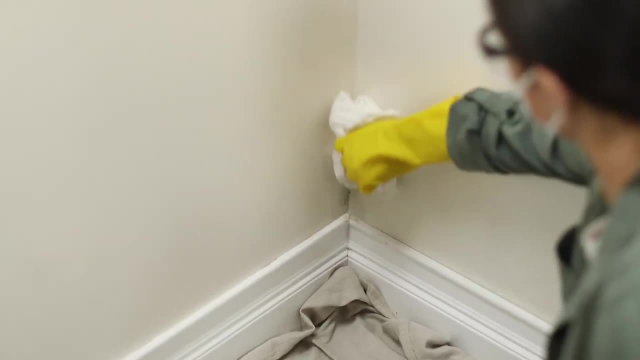 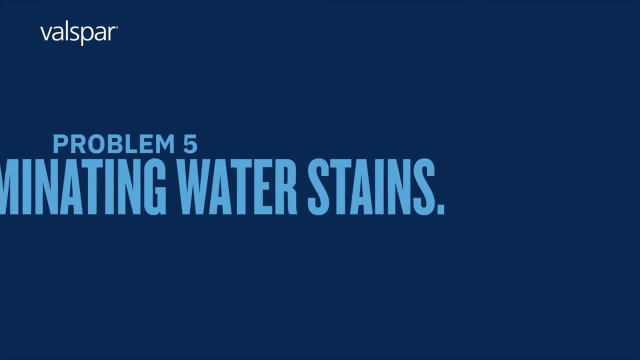 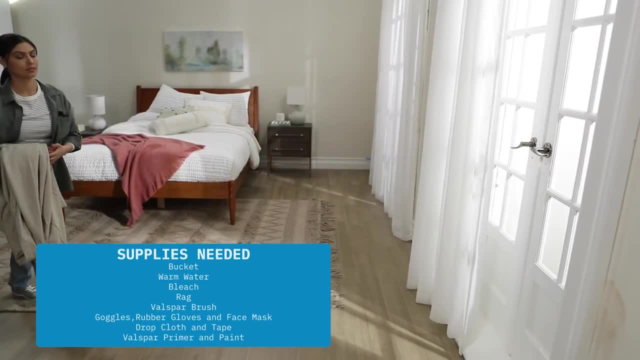 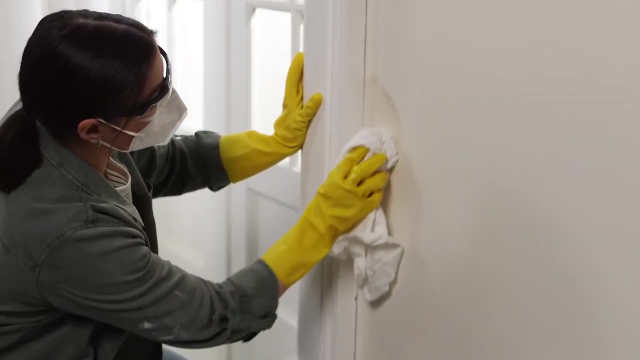 solution. First make sure that the water or leak issue has been resolved. then start by scrubbing with a one-part bleach to three parts water solution. Wait until the affected area is as dry as possible. We recommend using a dehumidifier, if it's available to you Then. 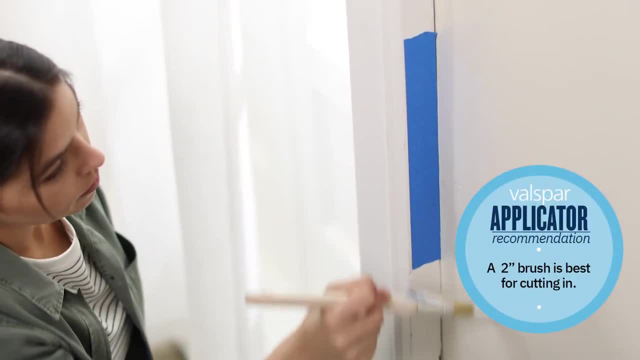 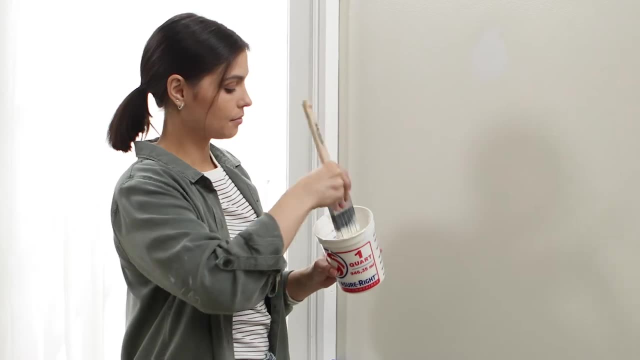 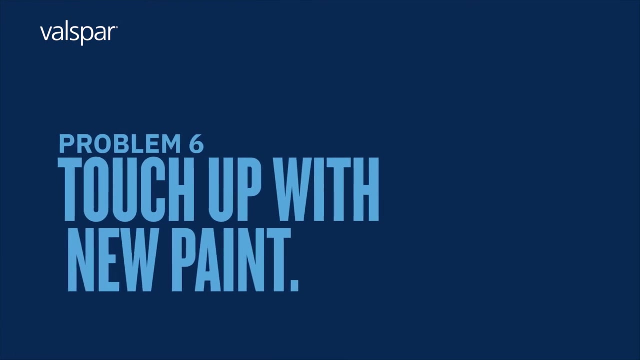 apply an appropriate primer to completely cover the stained area to prevent the stain from bleeding in the future into your top coat. Finally, you can apply your paint. We recommend applying a second coat of paint to make sure the stain is completely covered. Walls naturally wear down in a lived-in space.